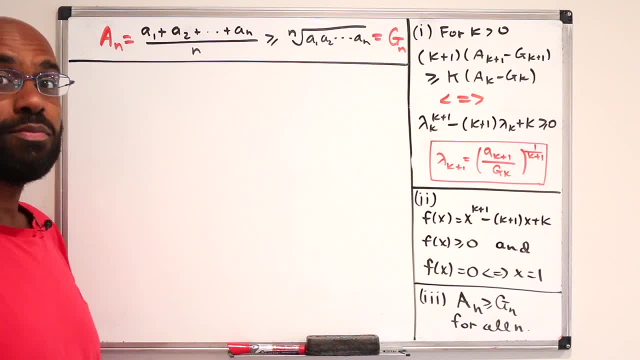 product of the number. The proof we're going to follow is outlined in Cambridge step 3 exam 2018, number 5.. So what I want to do is start by discussing the different steps so that, if you want to try this yourself, you can, and then we'll discuss the solution. So the first step is to make 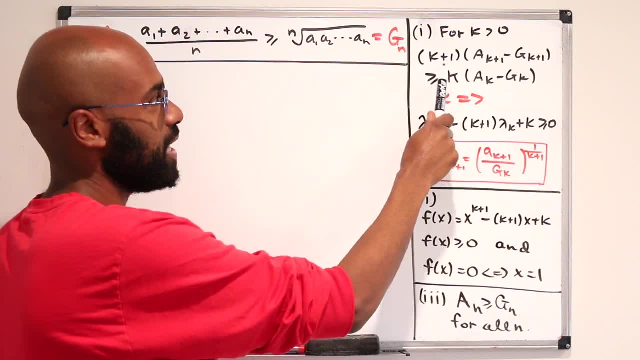 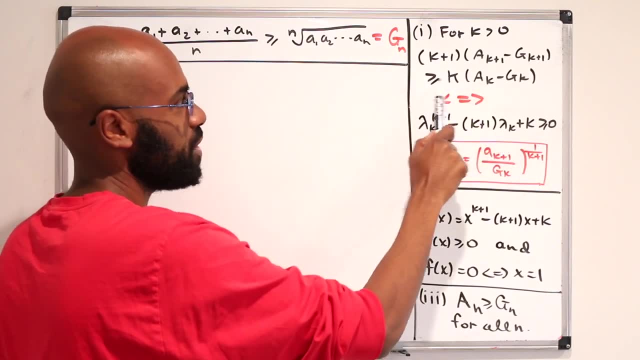 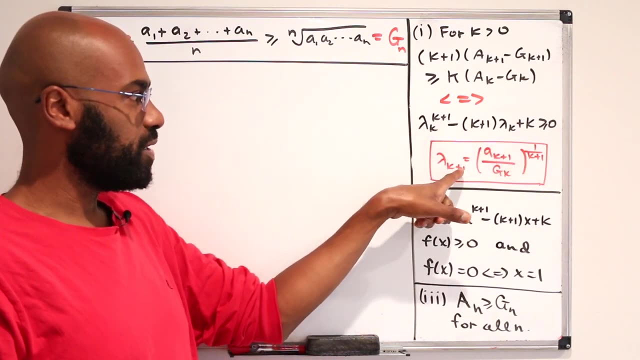 a relationship between the following expressions: that k plus 1 times the difference of the k plus 1th iterate of the arithmetic mean and geometric mean is greater than the k times the kth iterative of that. if and only if, you have this inequality satisfied by this quantity right here. 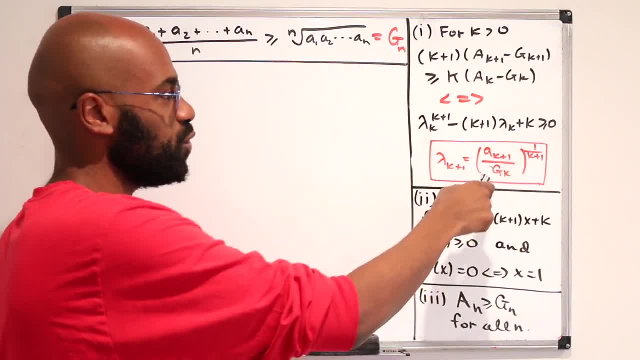 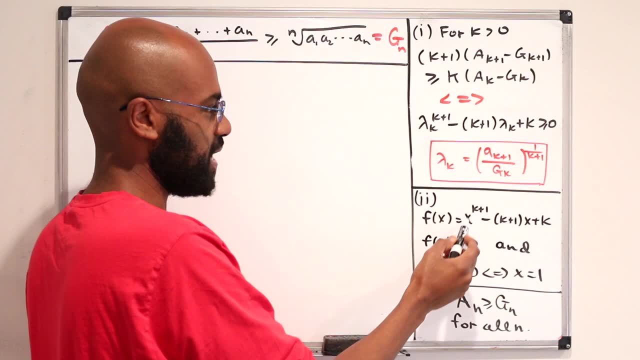 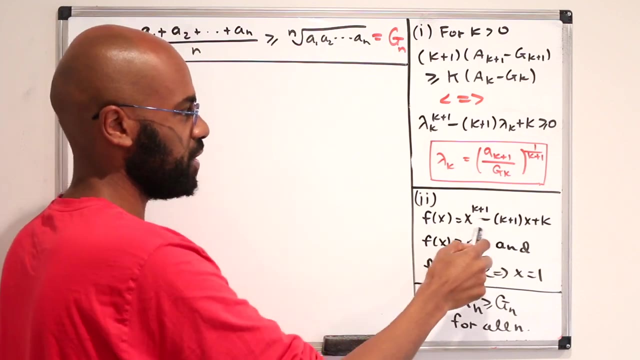 which relates the k plus 1th element of the sequence to the kth geometric mean. Now you can think about this as plugging in lambda k into a function. That function is x to the k plus 1 minus k plus 1, x plus k, and then establishing that that function is actually. 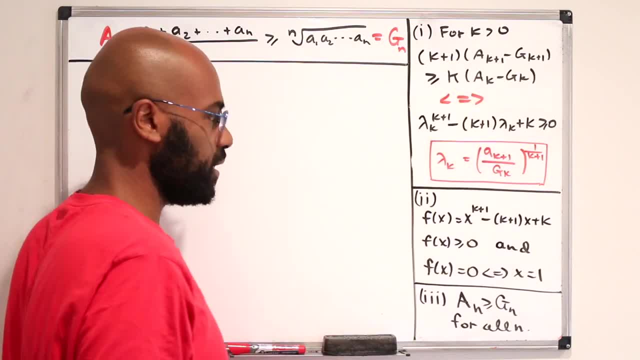 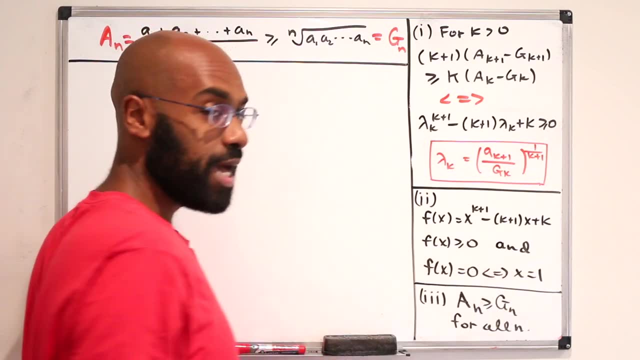 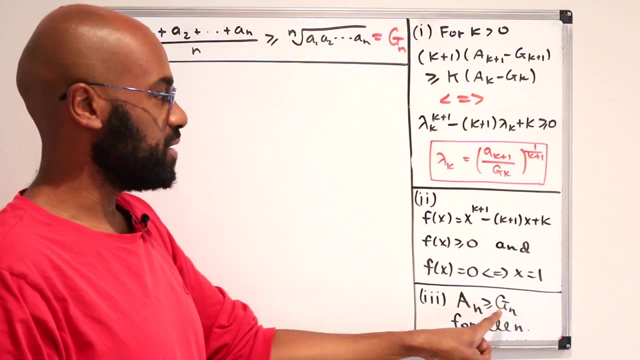 non-negative. So if you get the non-negativity, you get this inequality right over here. Now the non-negativity happens and the function is actually zero only when x is one, and you can use that, combined with what you prove here, to piece together that you have this. 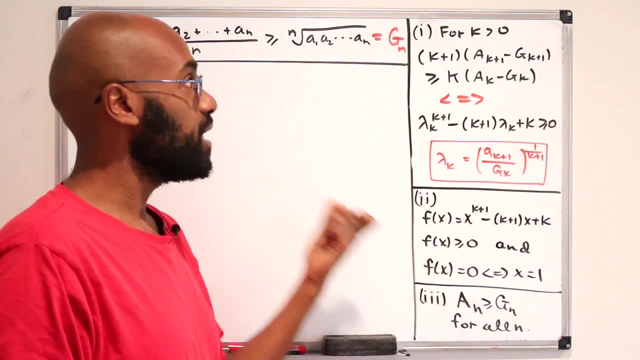 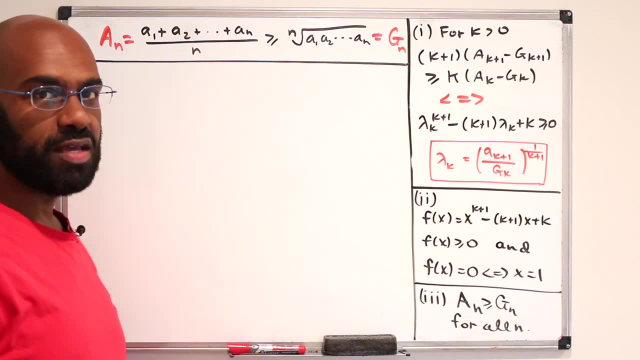 inequality and to show that equality holds if, and only if, all of the entries of your sequence are actually equal. It'll be beneficial for us to think about our sequence as an infinite one, consisting of positive numbers- a1, a2, a3, etc. onward- and then thinking about 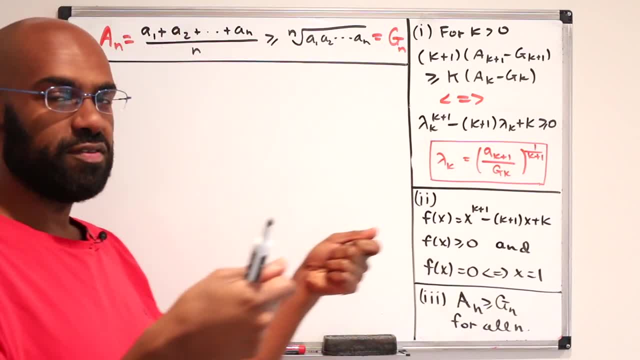 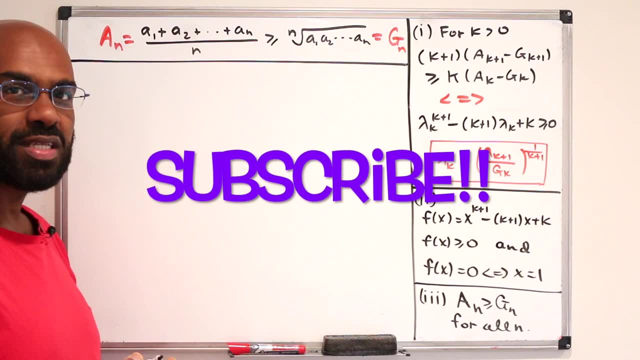 the arithmetic mean and geometric means as two sequences of numbers indexed by the natural numbers n. Okay, so if you want to pause the video, give this a try, trying each of these steps, and we'll discuss the solution. So first let's look at part one. I'm going to start with 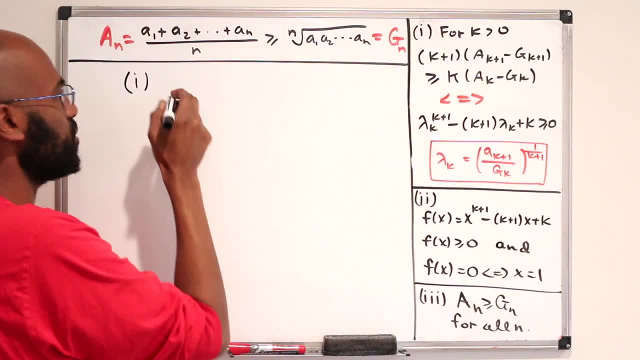 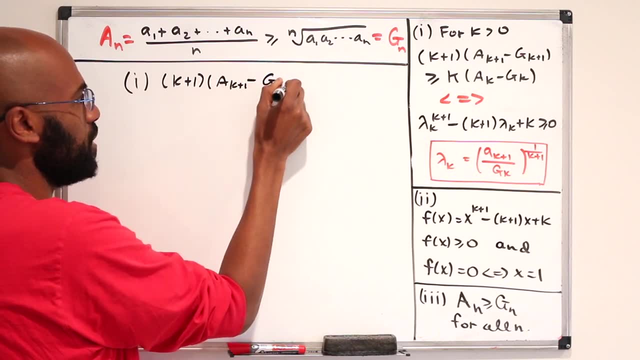 this expression and what I'm going to do is rearrange it so that this is on this side. So, looking at the expression k plus 1, a k plus 1 minus g, k plus 1 minus k, times a k minus g k. Now, 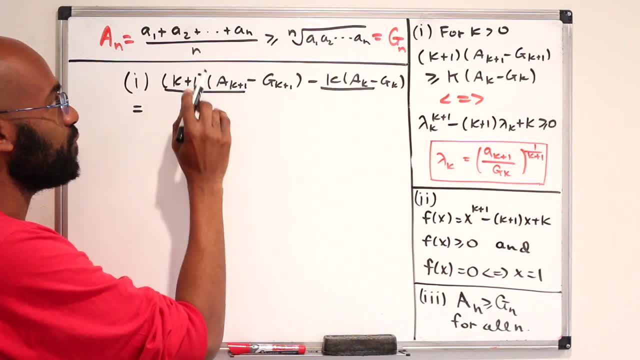 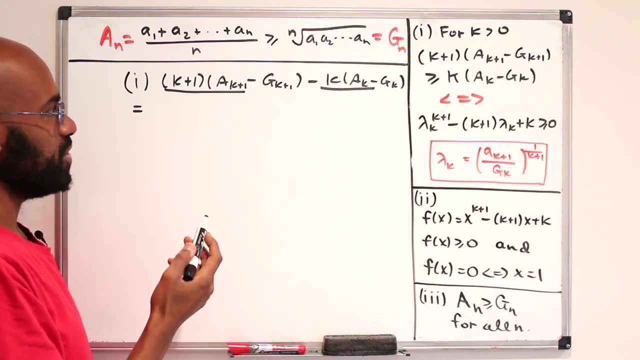 k plus 1 times a k plus 1 is the sum of the first k plus 1 numbers in our sequence. Similarly, k times a k is the sum of the first k entries in our sequence. So if we pair these two things together, we're going to be left with a k plus 1 itself. 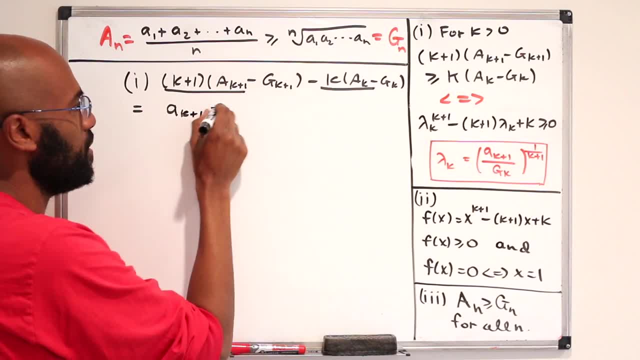 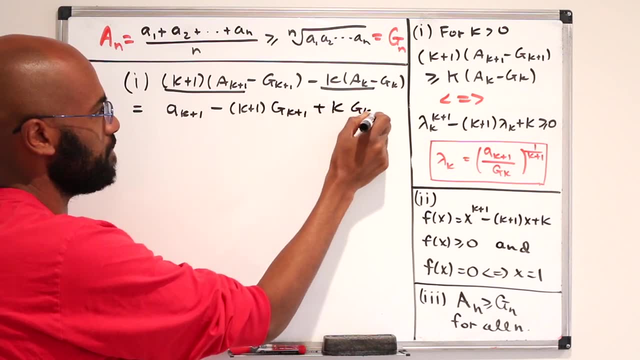 Alright, and then that leaves us with minus k plus 1 g k plus 1 plus k g sub k. Alright, so we're trying to prove that this is greater than equal to 0, if only if. this is So, let's start by saying that this: 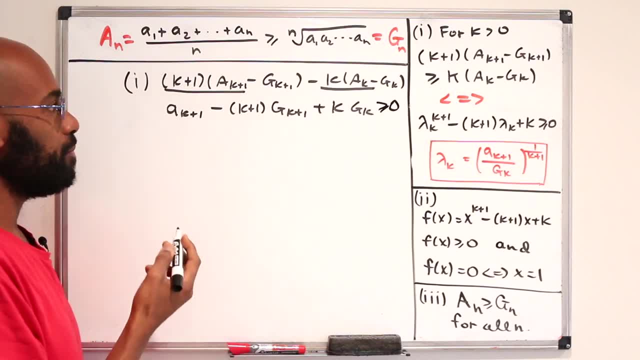 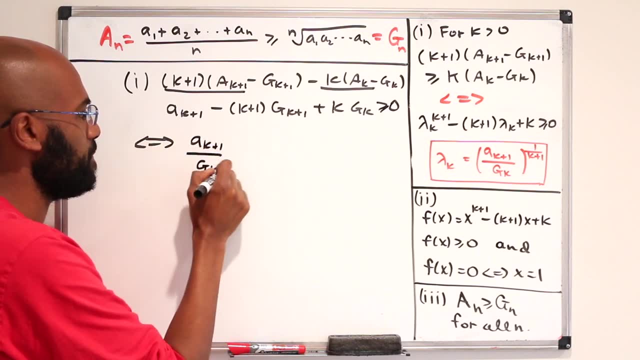 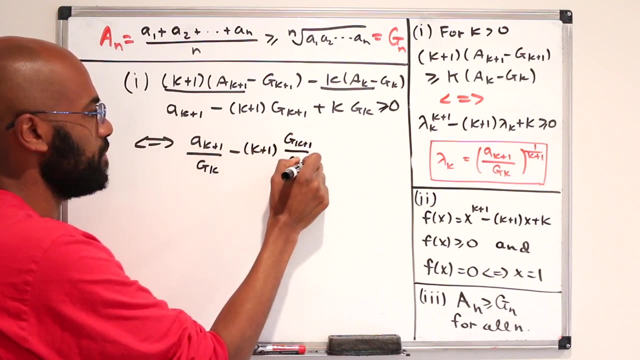 is greater than equal to 0.. Since g k itself is a positive number, this is true if, and only if, a k plus 1 over g k minus 1 times the quantity g k plus 1 over g k plus k is greater than equal to 0 by dividing by g sub k. 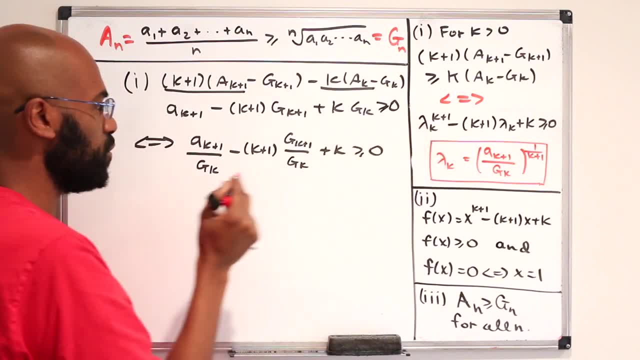 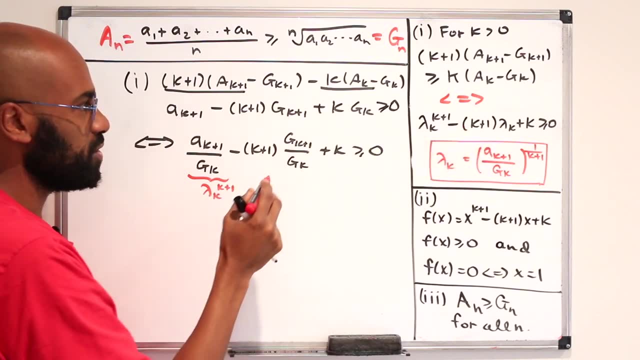 Okay. so you might notice something here. We have a lambda k to the k plus 1, and that's precisely this thing. right over here We have the k plus 1 coefficient like we do here. we have the k here, so it seems like this must be lambda k, and let's actually check whether or not that's the case. 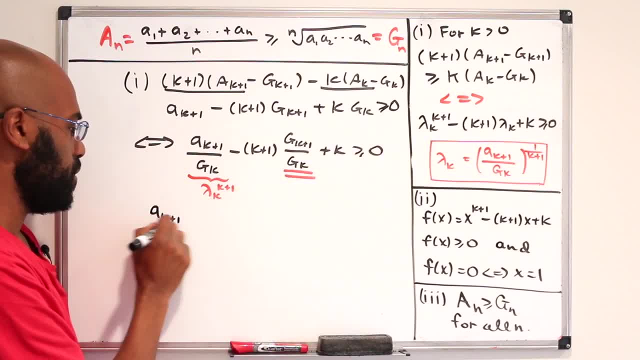 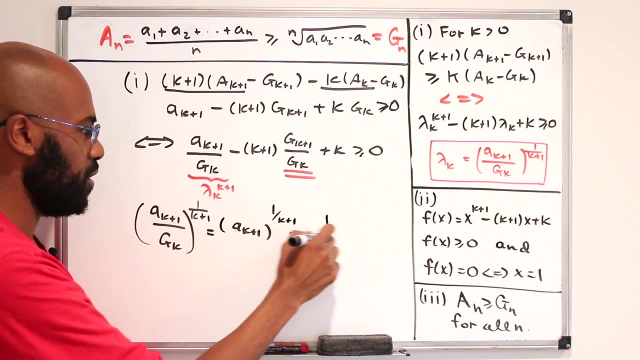 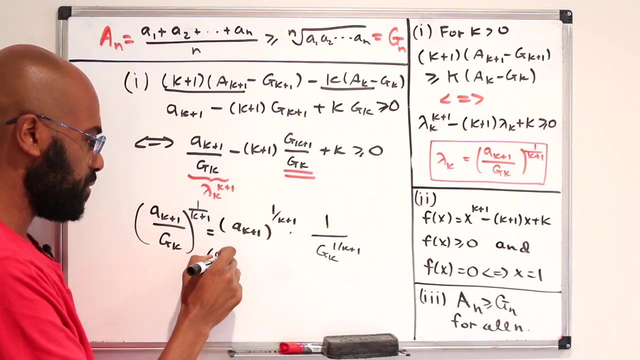 So we'll start with lambda k, that's a k plus 1 over g, k raised to the 1 over k plus 1, and we'll write it as a k plus 1 raised to the 1 over k plus 1 times 1 over g, k raised to the 1 over k plus 1.. Now a k plus 1 itself can be written as the product. 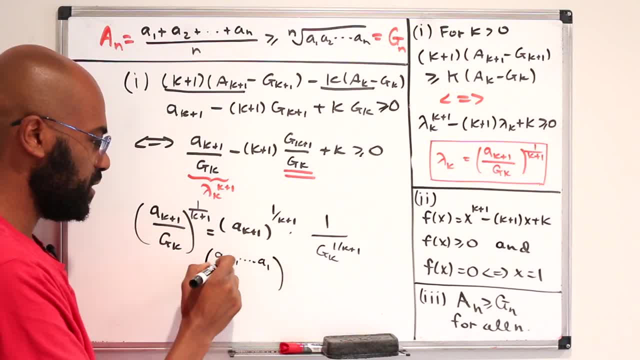 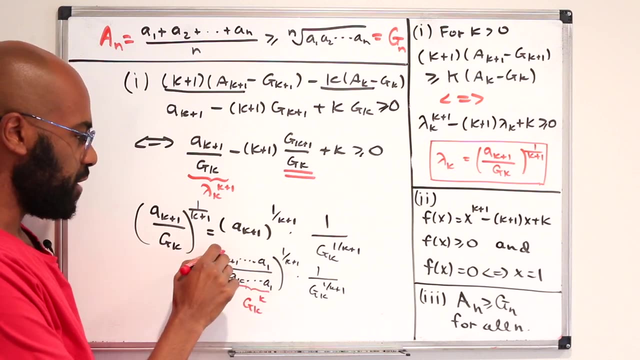 of the first k plus 1 entries divided by the first k entries and we have that raised to the 1 over k plus 1.. We still have this piece right over here Now. the denominator here is g k to the k and the numerator is g? k plus 1 to the k plus 1.. So in total we get g k plus 1 to the k plus 1. 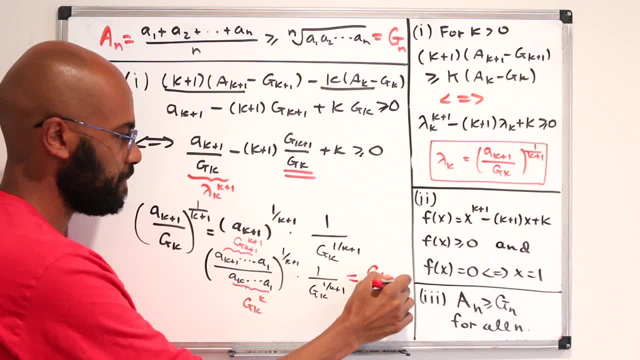 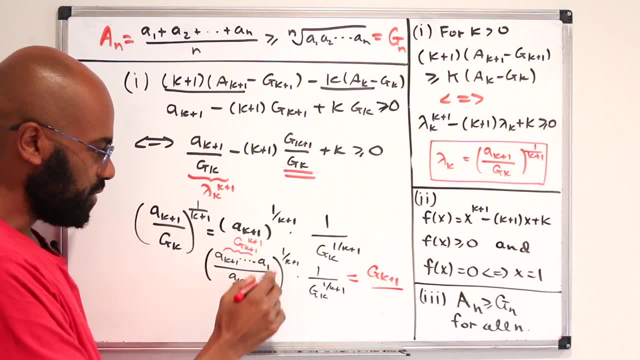 raised to the 1 over k plus 1, which is g k plus 1, and then in the denominator we have g k to the k raised to the 1 over k plus 1, right? so the exponent on g sub k in this whole thing is k over k plus 1. then we have this extra 1 over k plus 1, which gives us 1 as well. 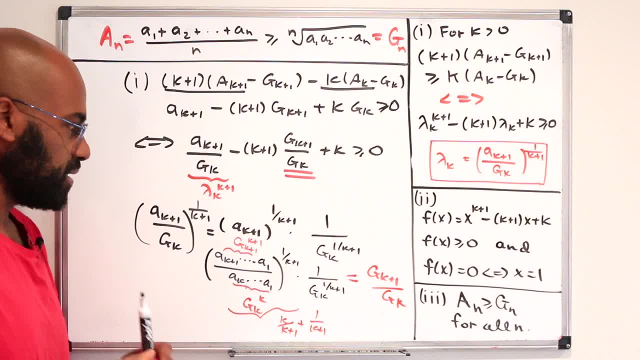 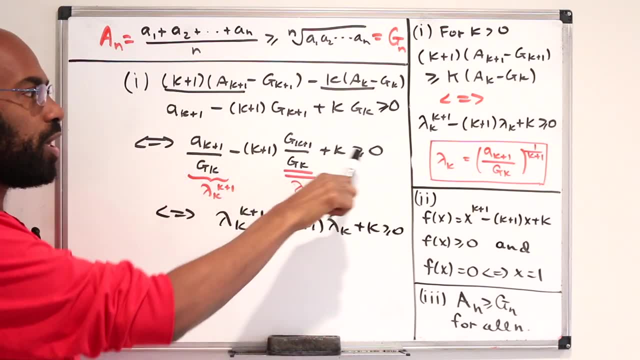 So the denominator we have g, k, so it is the case that this quantity is lambda k itself. So, subsequently, this inequality is the same statement as this inequality right over here, which is the inequality that we actually wanted Great. so this inequality does happen if and only 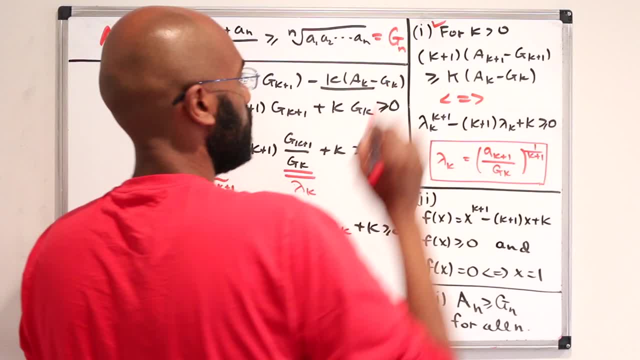 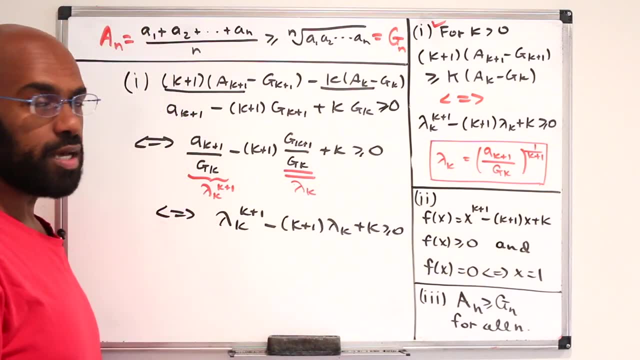 if this one does, And so we've dealt with this first part of the problem. Now let's analyze this function and look at when it's non-negative, why it's non-negative, and use that, together with these conditions, to determine why our inequality is true. 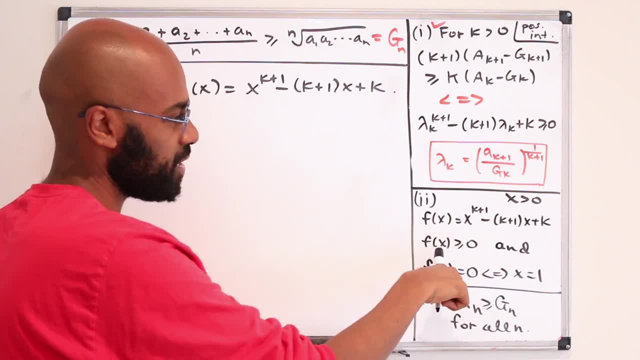 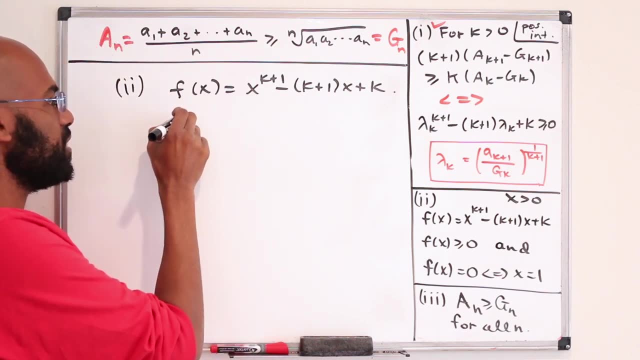 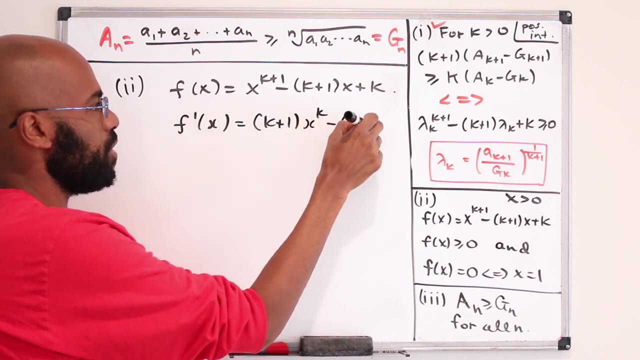 Okay, so now let's analyze this function here and prove that it's non-negative and it being 0 if, and only if, x equals 1, using some calculus. So let's differentiate first the derivative of this function. So the derivative of this function is k plus 1, x to the k minus the quantity, k plus 1,. 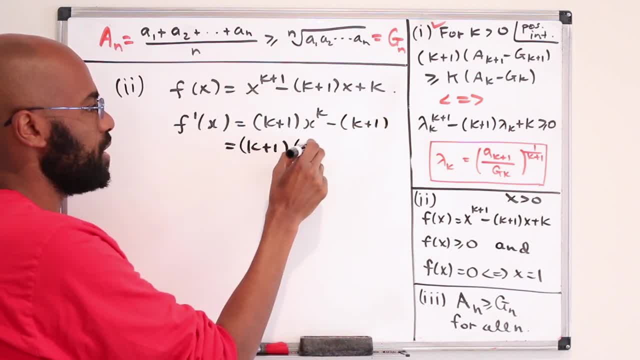 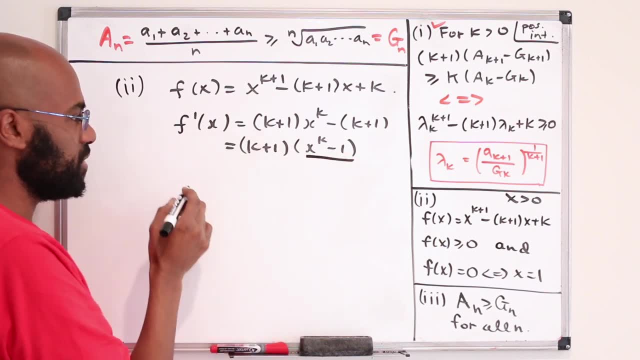 which we can factor into k plus 1 times the quantity x to the k minus 1.. Critical points happen when this function is 0, and that happens only when x is 1.. So we get a critical point at x equals 1.. 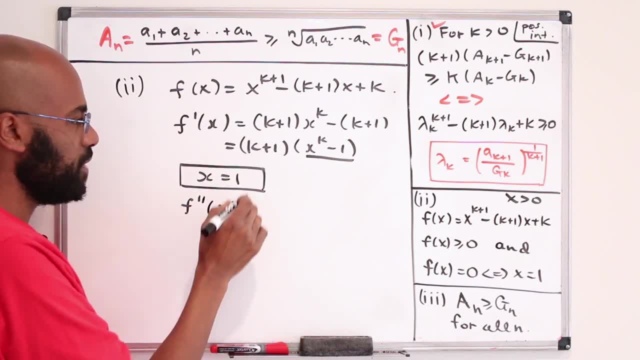 Now, to classify that critical point, we need to take a second derivative. The second derivative is k plus 1 times k times x to the k minus 1.. And so f double prime at 1 is a positive number. It's this product right over here. 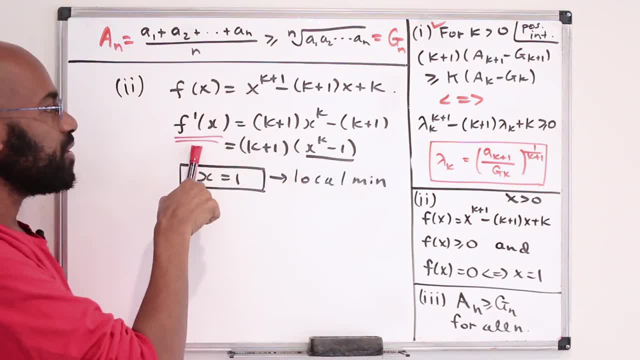 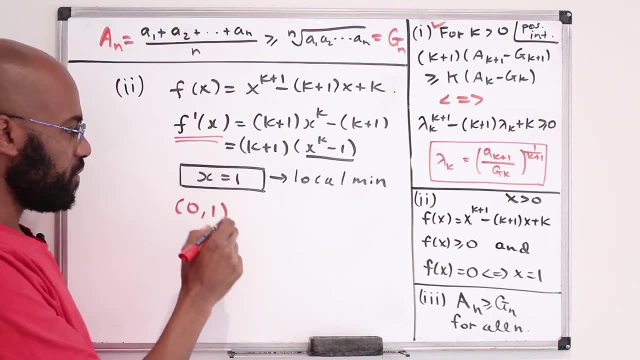 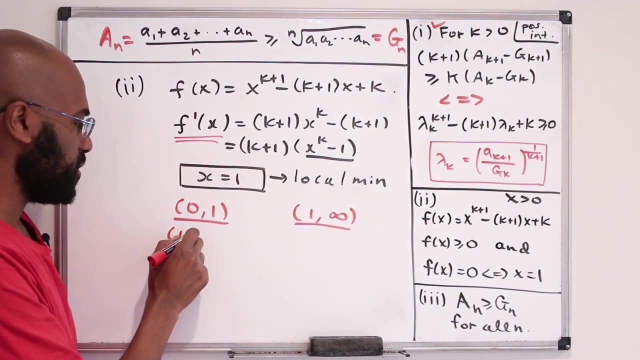 And so this thing is a local minimum. Now let's look at the first derivative to get a sense of what's happening with the actual function. So we have two regions: One is before this critical point and one is after this critical point. Before this critical point, our derivative looks like k plus 1, x to the k minus 1.. And since x is, 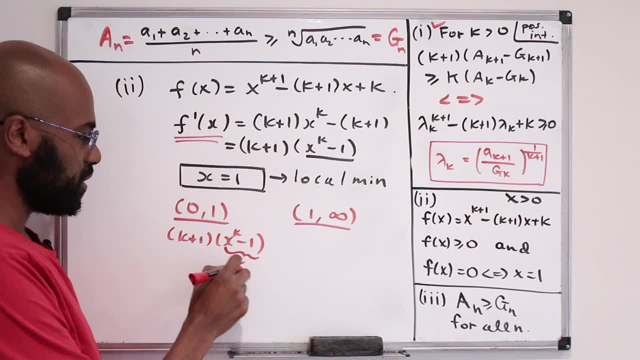 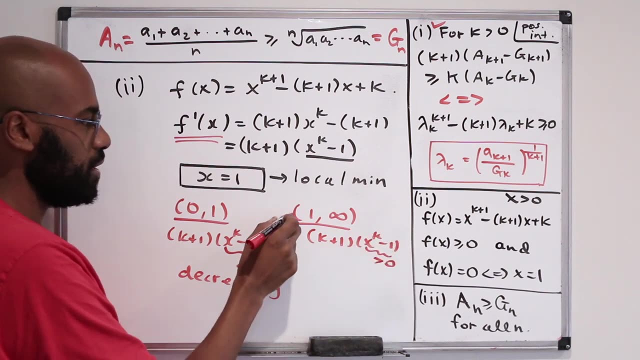 between 0 and 1. this value here is going to be strictly less than 0. So we'll have that the function is decreasing on this interval. Now, in a similar light, this quantity here is going to be greater than 0 in the interval 1 to infinity. so this function is increasing here. 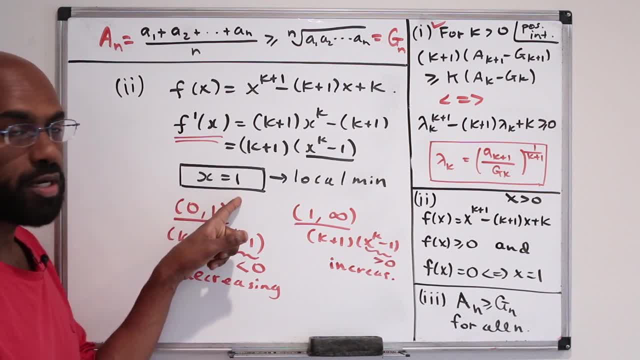 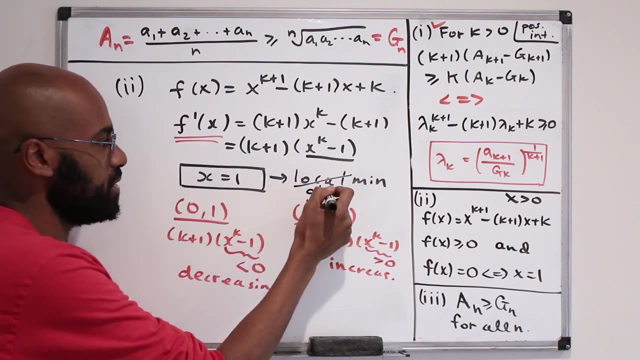 All right. so we have this function and we have a local minimum at x equals 1.. The function decreases to that local minimum and then increases afterward. So that means that this local minimum for x greater than 0 is actually a global minimum. Right, it is the minimum of the function. 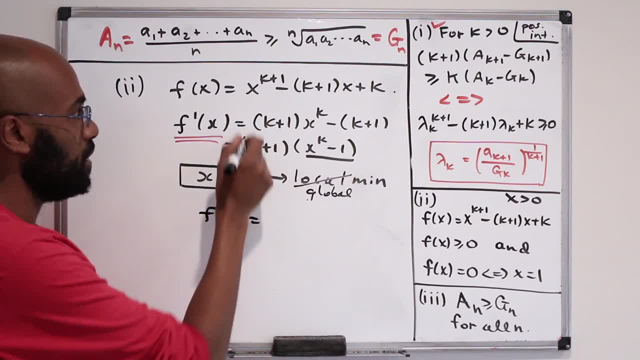 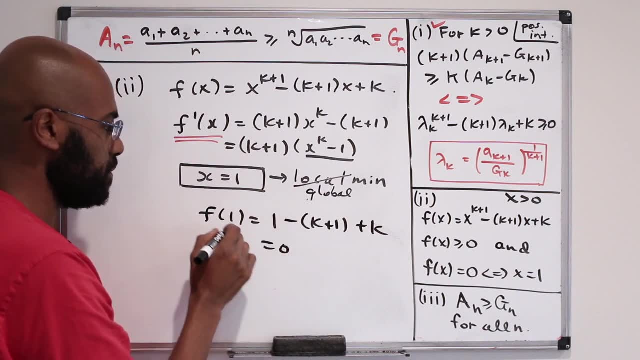 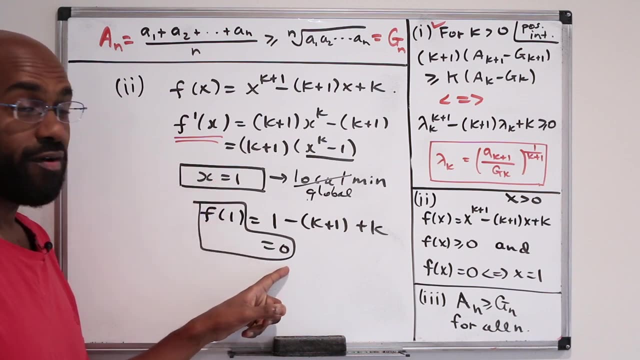 Now the actual value of f of 1 is 1 to the k plus 1 minus k plus 1 times 1 plus k, which is 0. So we have that this function has a global minimum at x equals 1 with a value of 0. So the function itself is greater than equal to this value: 0. 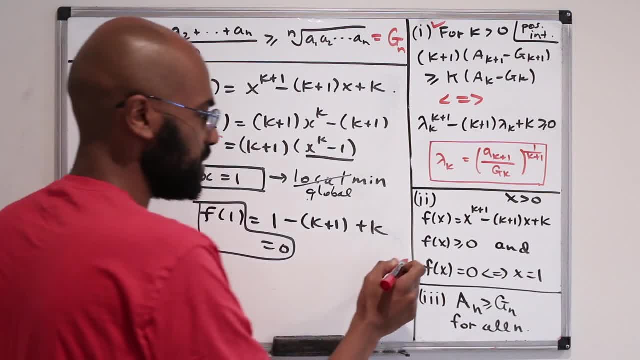 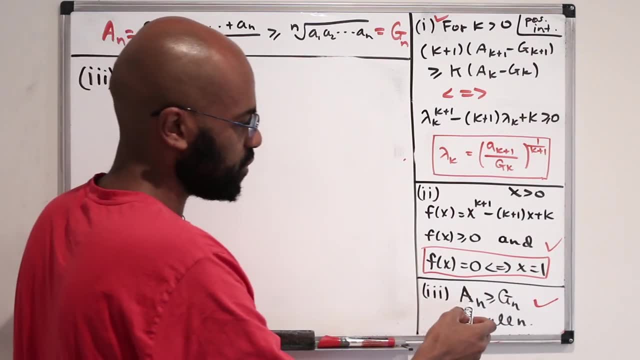 and equality happens only when x is 1, and that's exactly the thing that we were trying to prove, So we're happy. Okay. so the final thing for us to establish is why n is greater than equal to gn for all n. So we're going to exploit this inequality right over here. 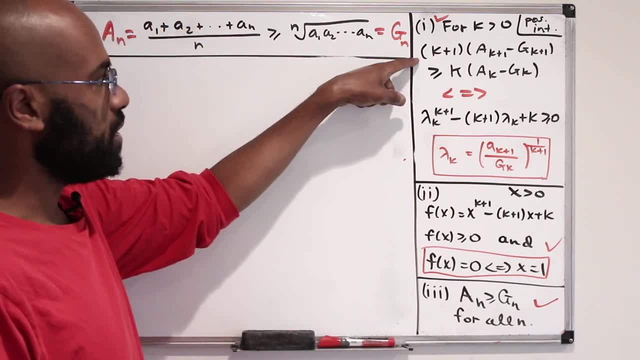 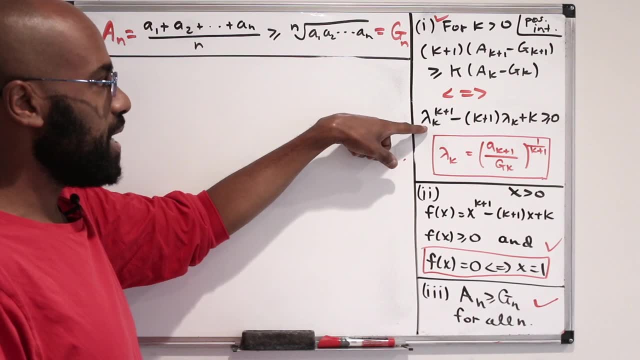 and lucky for us for any k. this inequality is going to hold no matter what. And the reason is this happens if, and only if, this happens right. And then we establish that this actually does happen because this function is non-negative for positive values of x. 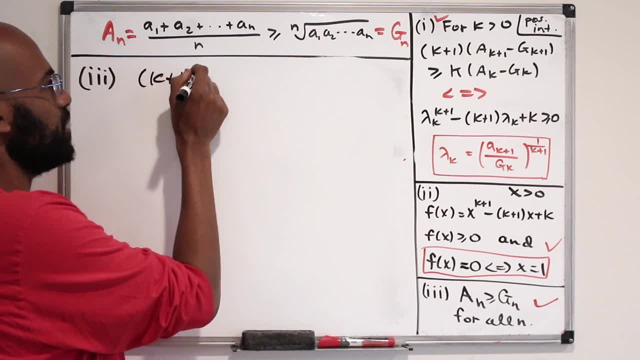 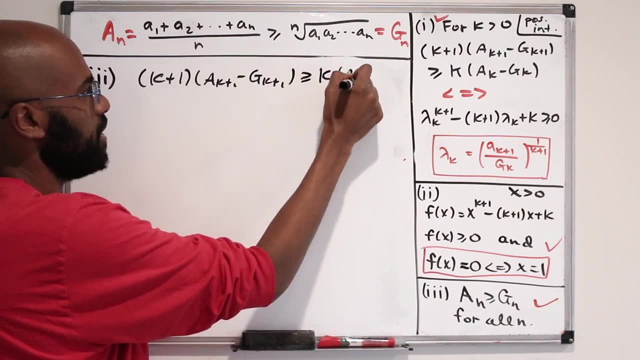 Okay, so we have that k plus 1, a k plus 1 minus g, k plus 1 is greater than or equal to k. a k minus g, k for all k. Okay. so first of all, we want to be able to calculate the real equation for n for all, a minus 1.. 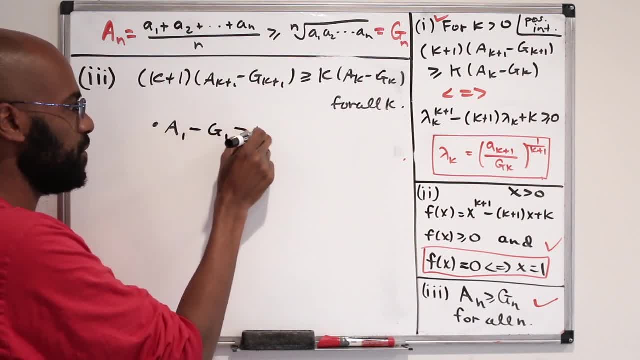 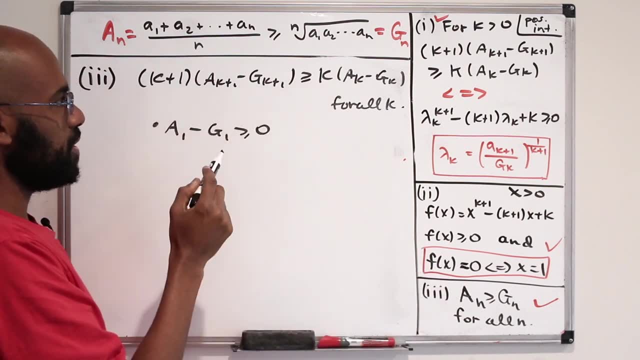 we actually know that a1 minus g1 has to be greater than or equal to 0. They're actually equal. They're both equal to a1 itself. Okay, so you can think about this process, then, as being inductive. So if you assume for some k that ak minus gk is greater than or equal to 0,, 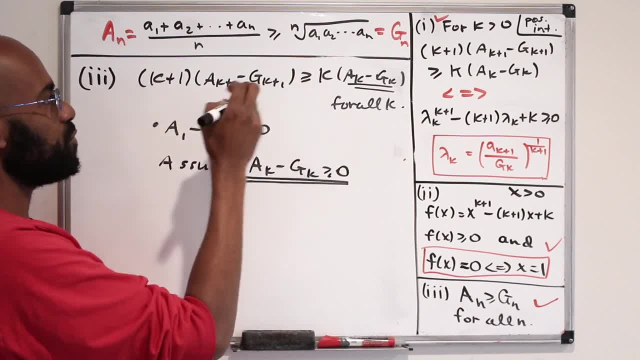 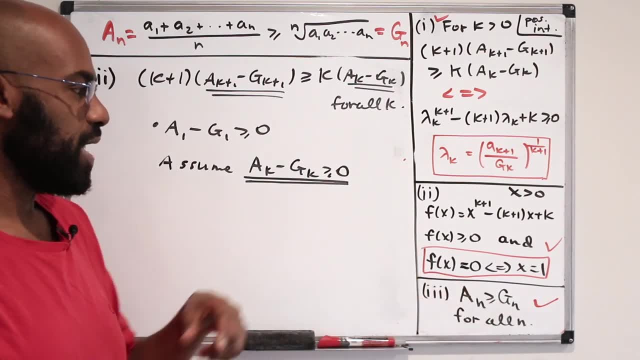 then this quantity here would be greater than or equal to 0. And if you divide by the k plus 1, you get that this quantity here is greater than or equal to 0. So we have this cascading effect that allows us to show that an is greater than or equal to gn for all n. 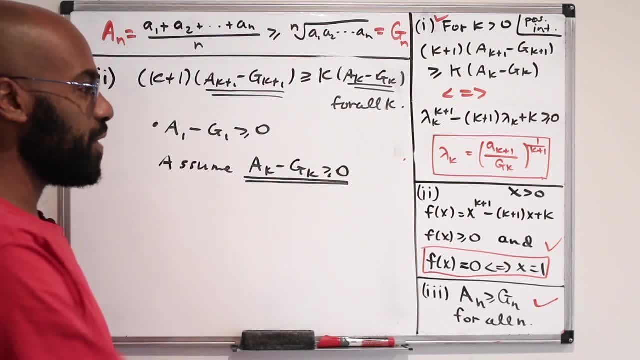 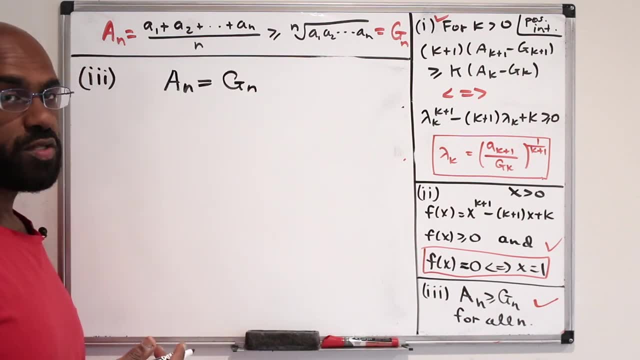 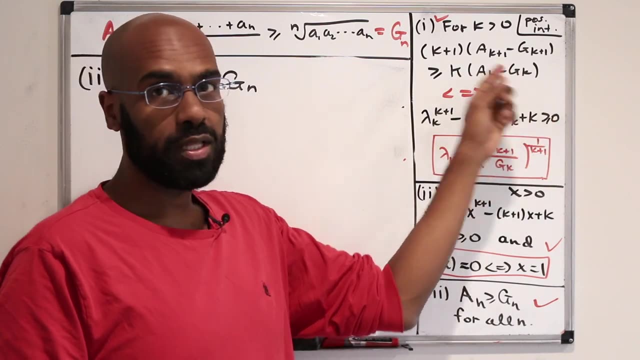 Now we can actually take this a little bit further and show that equality here holds if, and only if, all of the a sub i's are equal. To do this, let's say that an equals gn for some particular n. Now we know that the right-hand side of this inequality is non-negative. 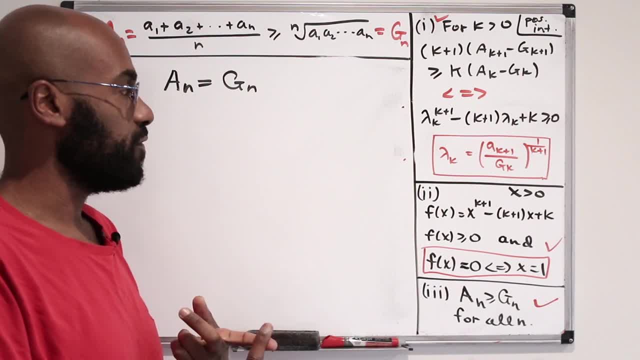 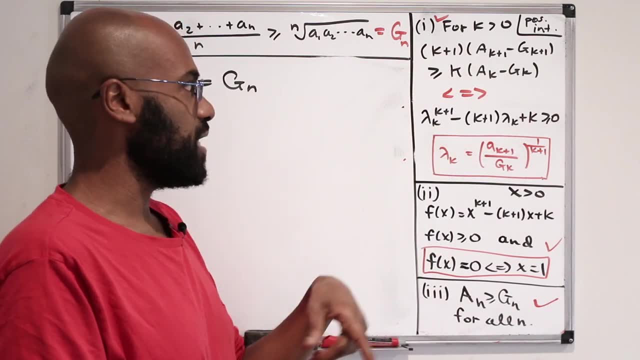 The reason is because a1 minus g1 itself is non-negative, And then you can iterate this inductively to get that this expression on the right-hand side is actually non-negative. For example, if you wanted to know that a2 minus g2 is non-negative, 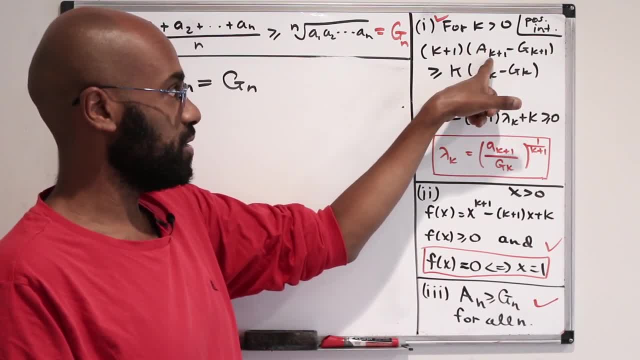 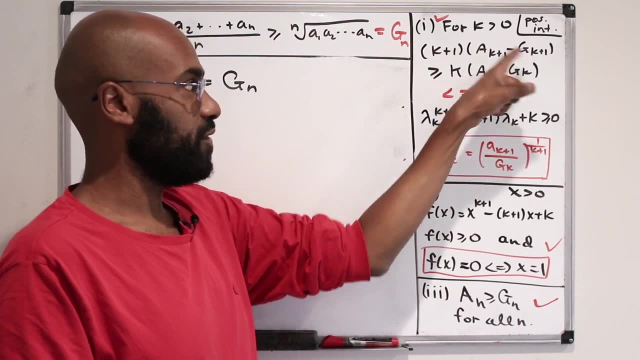 you know, a1 minus g1 is non-negative, And so from this, a2 minus g2 is non-negative. And then when k equals 2, you get: because a2 minus g2 is non-negative, a3 minus g3 is non-negative, etc. 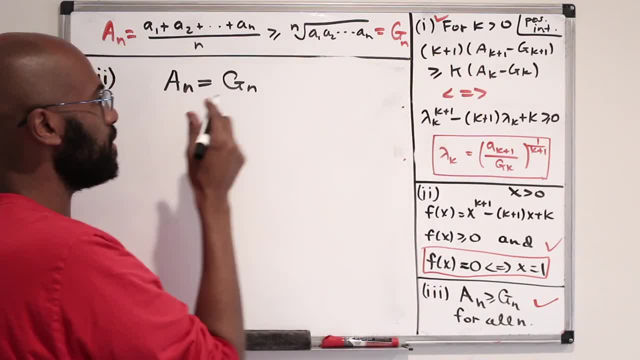 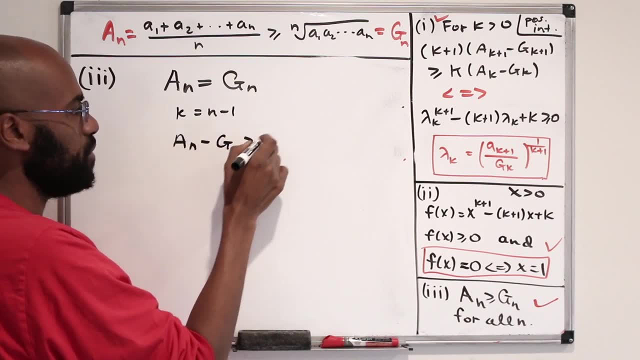 So the reason this matters is because if you have an equal to gn, then plugging in k equals n minus 1 into here you get an minus. gn is greater than or equal to n minus 1 over n, because the real amber, the real f. 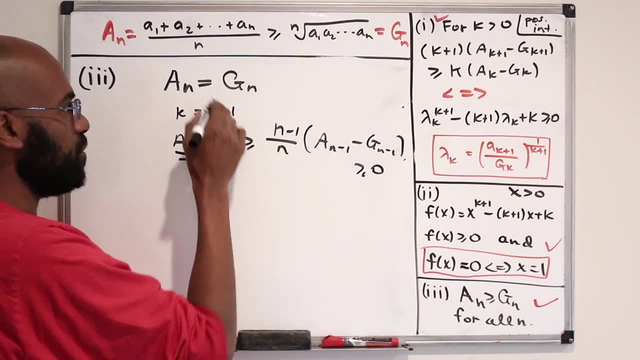 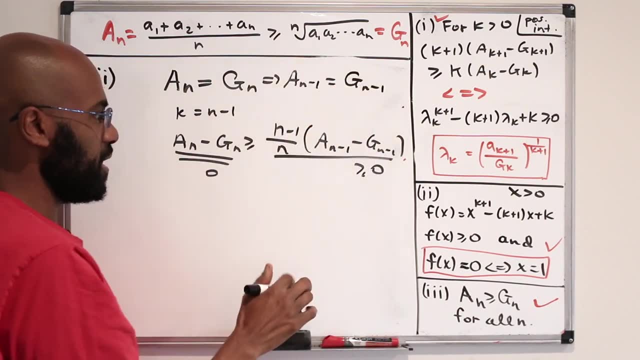 you know this is lowest grade one. all these points are also not minors. equals to n minus 1, plus g is no minus 1.. So this Mount is actually n. so I get a n minus 1 times a n minus 1, g, n minus one. 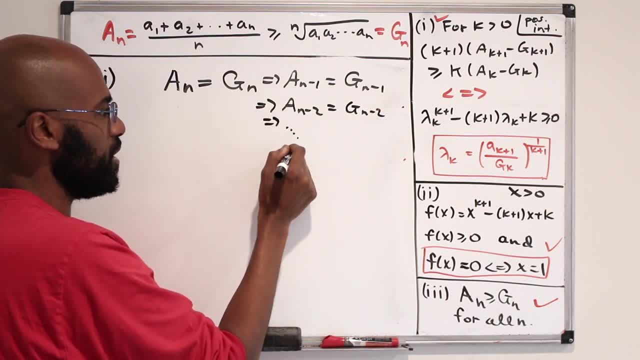 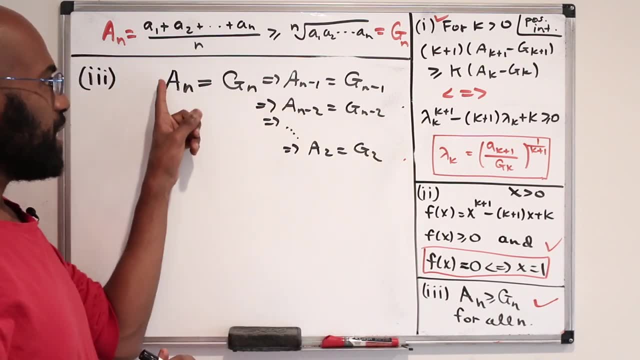 which is non-negative, but this thing actually is zero. these are equal, so this implies this quantity here has to be zero, So that means a n minus 1 already. So now, if we have all of these being equal, then these expressions are: 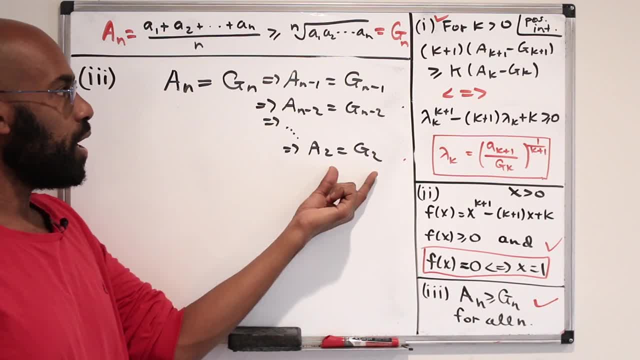 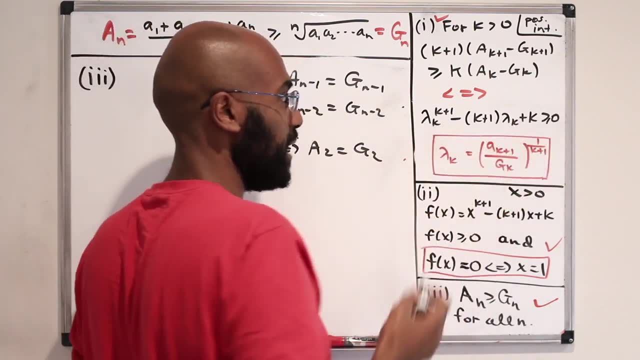 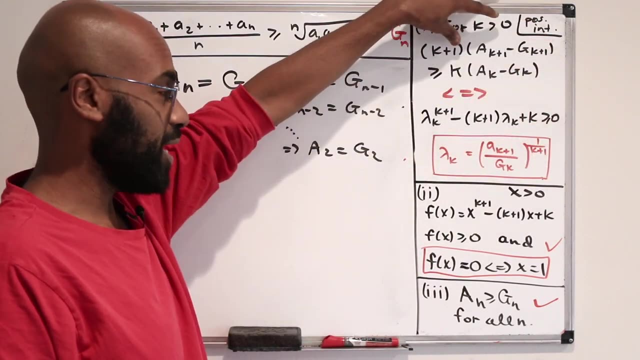 all 0 for k between 1 and n minus 1.. This being equal to this actually means that this expression on the left is 0, because when we rearrange this expression to have 0 on the right hand side, that expression actually identically is this expression right over here. Okay, but the only way that. 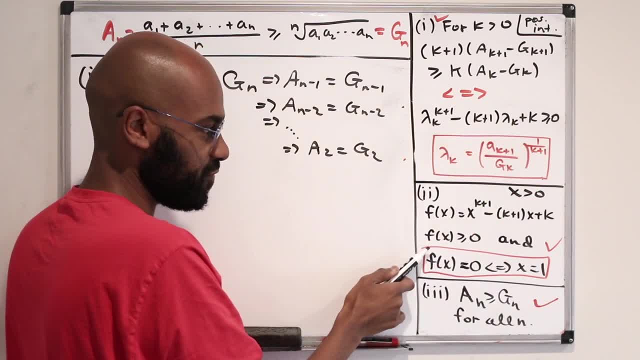 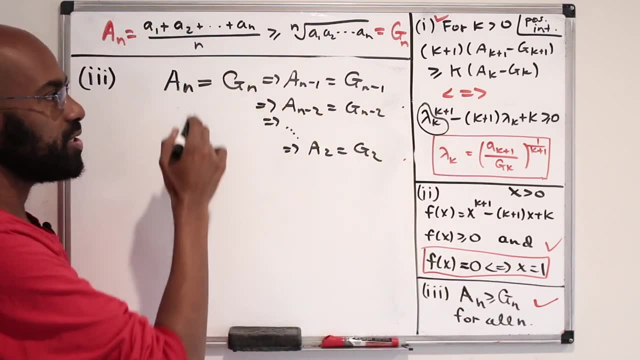 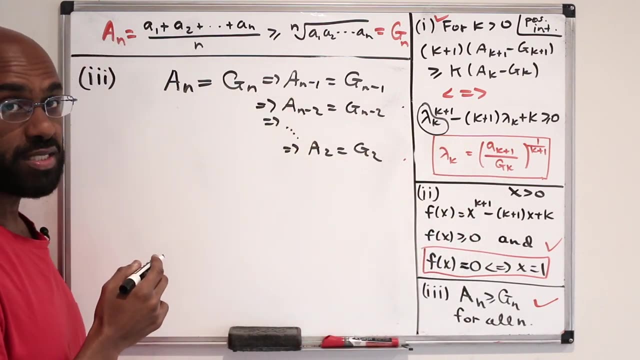 this expression is 0 by our analysis from here is if this lambda k itself actually equals 1.. So as a consequence from this, we get that all of these lambda k's are 1, for k equal 1 up to n minus 1, so let's analyze what that. 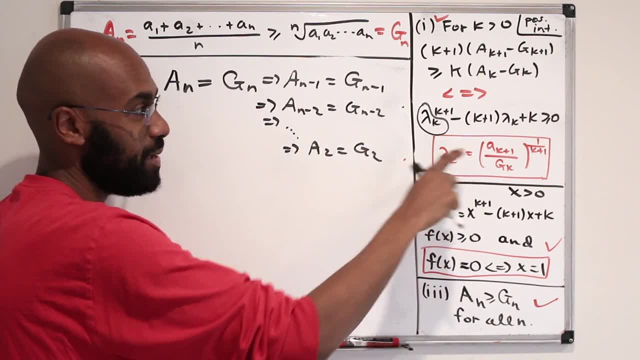 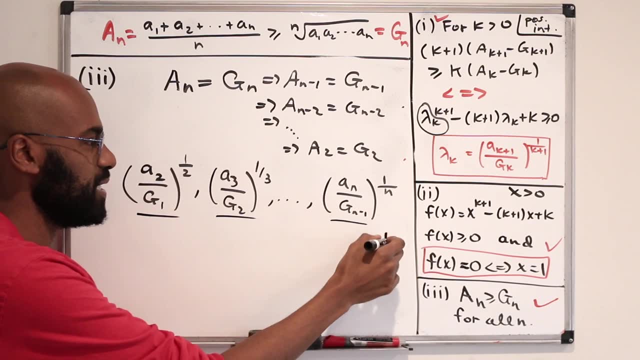 tells us. So first of all let's write down what the expression lambda k is per k from 1 to n minus 1, so by our analysis, all of these expressions have to identically be equal, so we actually have that expression into the first. 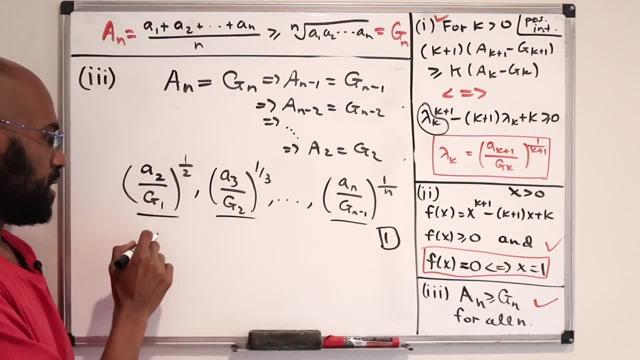 two expressions as a professor, So as a peeve for you, and your happens to do be 1.. So let's look at this part right over here. If this is 1, that means that a2 is the square root of a1. a2, because this expression here is 1.. And if we square, that means that a2 squared is a1. 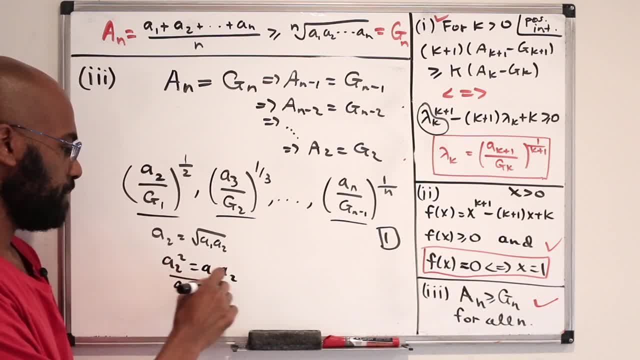 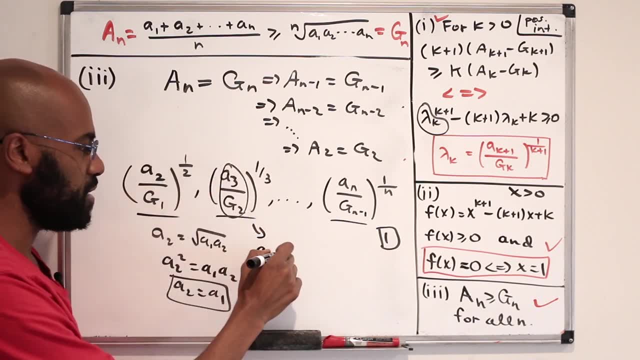 a2, and so a2 is a1.. Great, Now let's look at this expression. This here has to be 1.. That tells us that a3 is the cube root of a1, a2, a3. Cubing, we get a3. cubed is a1, a2, a3. And since a1 and a2 are, 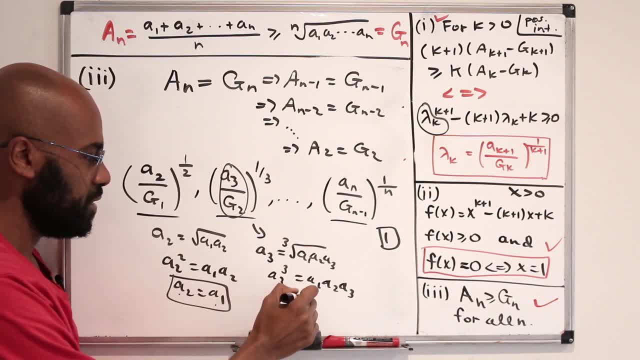 the same. this tells us that a3 cubed is a1 squared a3. Dividing by a3, we get a1 squared and a3 squared are the same. They're both positive numbers, so we can add a3 to the mix as being. 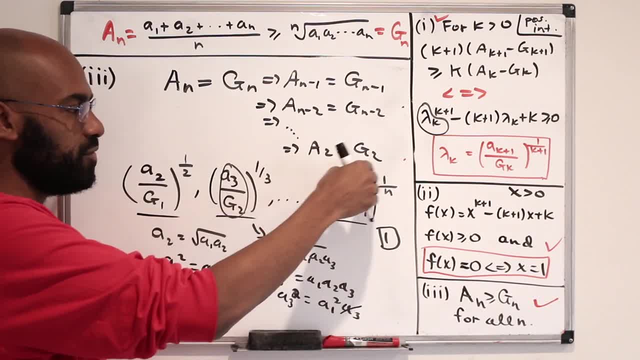 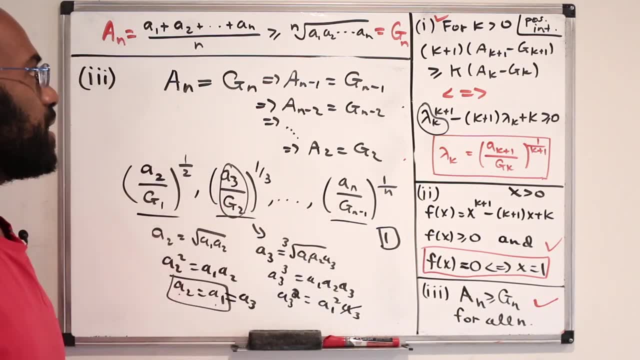 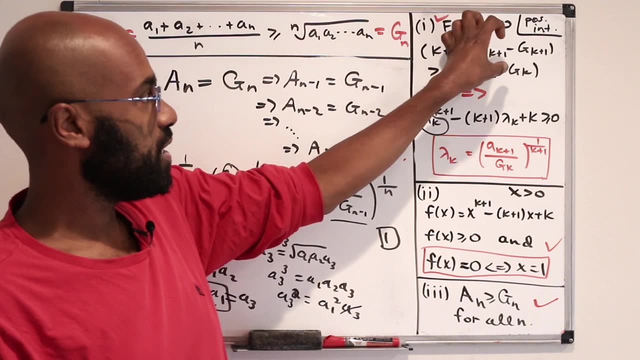 equal to all of these, And the same thing happens inductively, if we wanted to go about it rigorously, establishing that all the a i's are actually equal. So it's a cool way to prove the arithmetic geometric mean, inequality, and also establishing when equality holds, using this inequality paired with an. 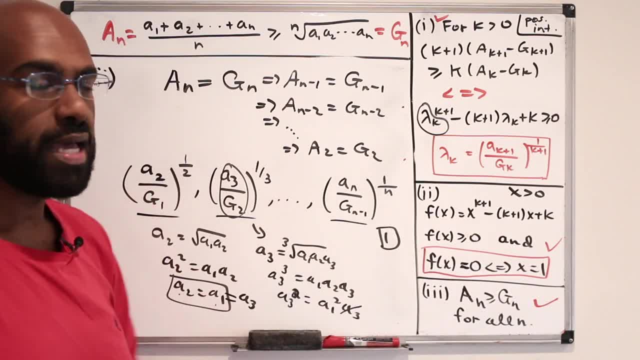 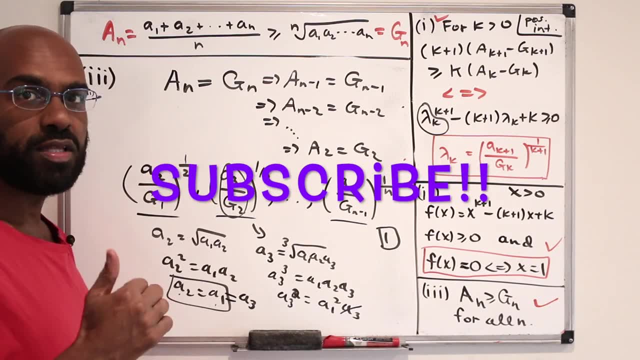 inequality. that allows us to use a function and calculus to understand when equality actually holds and why non-negativity holds. So I hope you enjoyed today's video. If you did, definitely click the like button. If you want to see more videos like this, subscribe to the channel.